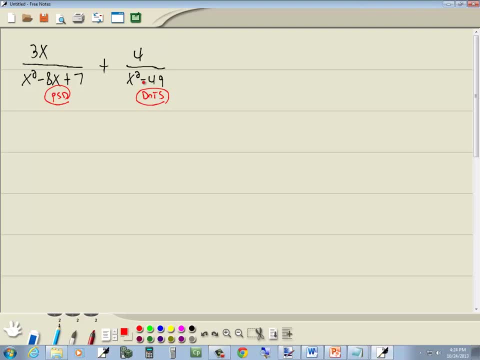 This next one is dots, because we've got two terms of myostringent, So let me go ahead and do these. So I've got x squared minus 8x plus 7.. Now PST: we take our number at the end, which is 7.. 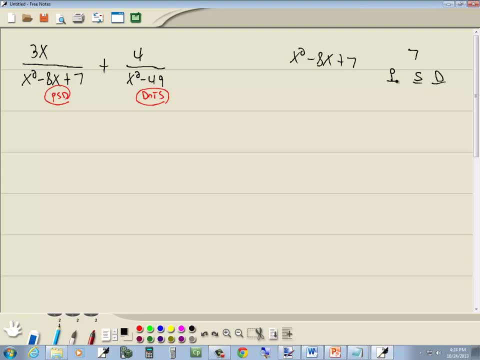 And we're going to create three columns: a P column, an S column and a D column. Now the P column, we list all the products to give us 7.. This one's primed, so it's pretty easy: 1 times 7.. 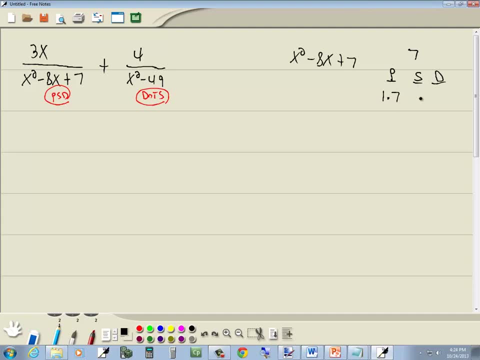 Now the S column. S is sum. We add these together: 1 plus 7 is 8.. D is difference Subtract smaller from larger. 7 minus 1 is 6.. The number we're looking for is the number in our middle term, which is 8.. 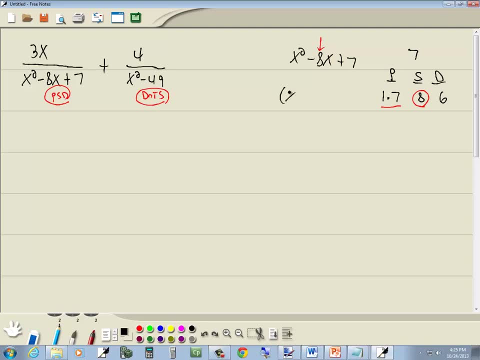 So we're going to use 1 and 7.. Now our larger number in the P column that we're using, which is this 7, is always going to be the same sign as the middle term, which, in this problem, is negative. 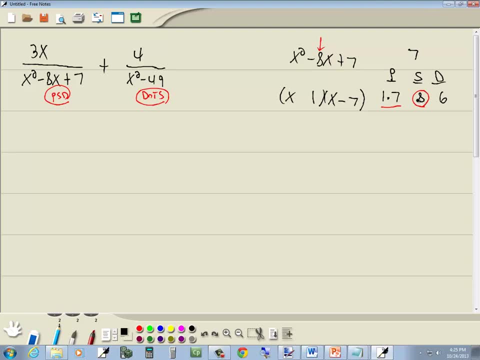 The number. I circled in the S column S, for same signs, or either both positive or both negative. Since this one's negative, then this one will have to be negative. So this first fraction factors as 3x over, x minus 1,, x minus 7.. 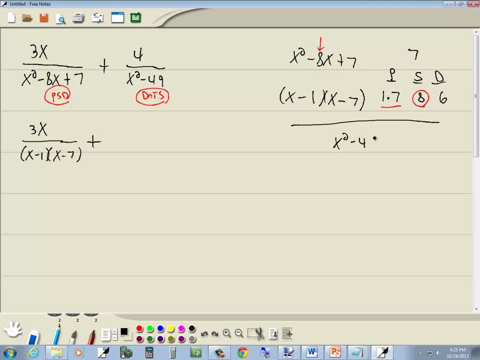 Now x squared minus 49.. The difference is 2 squares, Two terms of minus string it. We try to write it as something squared minus something else squared. You take a look at each individual piece and you ask yourself what times itself gives you that. 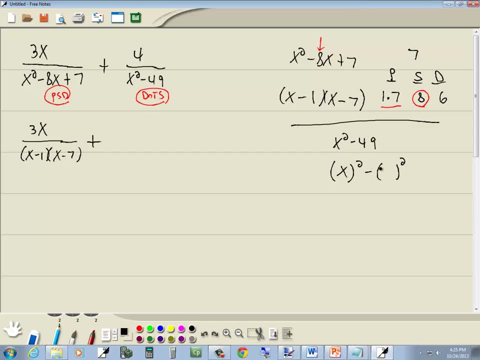 For the x squared, that'd be x times x. For the 49,, that'd be 7 times 7.. Now I'm going to label what's inside my first set of parentheses as f for first. I'll label what's inside my last set of parentheses as l for last. 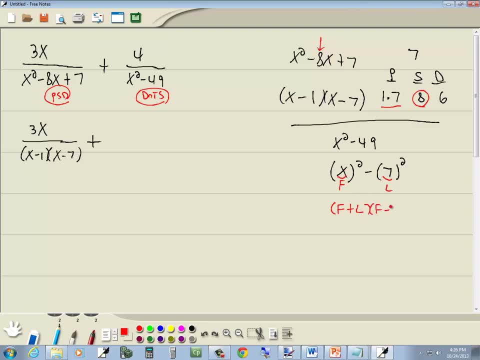 Our formula for the difference of two squares is f plus l times f minus l. Now, wherever there's an f, I'll plug in x, and wherever there's an l, I'll plug in 7.. So we've got x plus 7 times x minus 7.. 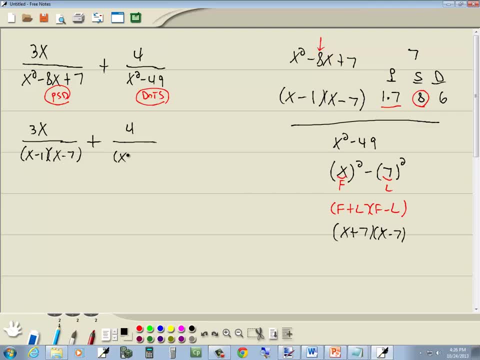 So this fraction becomes 4 over x plus 7, x minus 7.. Okay, next step: Figure out your LCD. We'll start with our first factor, the x minus 1.. Now I'm looking for the greatest number of x. 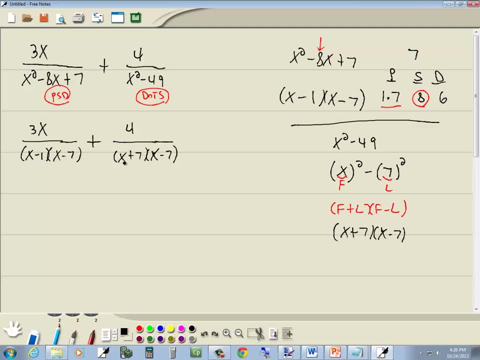 The greatest number of x minus 1 is in a single denominator. There's 1 here, there's none here. So the greatest number of x minus 1 is in a single denominator, is 1.. Now I go to my next factor, the x minus 7.. 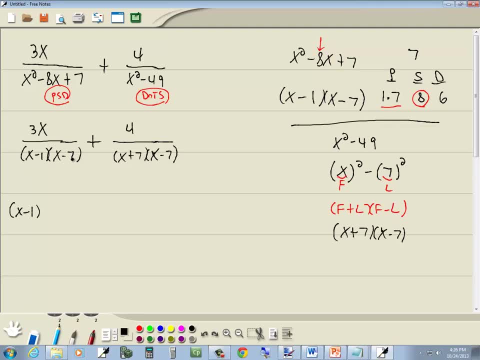 And I'm looking for the greatest number of x minus 7 is in a single denominator. Not counting how many there are, I'm looking for the greatest number in a single denominator. There's 1 here, there's 1 here. So the greatest number of x minus 7 is in a single denominator is 1.. 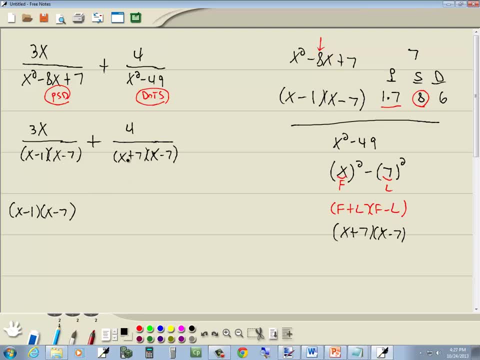 Now I go to my next factor, the x plus 7.. And I'm looking for: the greatest number of x plus 7 is in a single denominator. There's none here, there's 1 here. So the greatest number of x plus 7 is in a single denominator, is 1.. 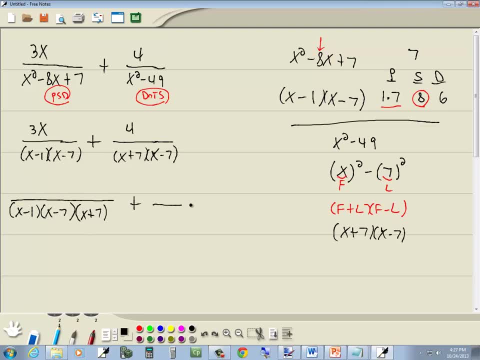 So that's our LCD. Now I want to rewrite each fraction with that new denominator. Okay, let's analyze this. We had an x minus 1, x minus 1 is still there. We have an x minus 7, that x minus 7 is still there. 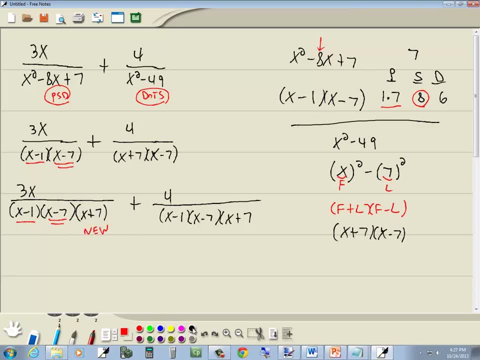 The new item in our first fraction is the x plus 7. So we have to put it up on top also. So again, you're looking for the new item downstairs And then whatever's new you have to also put up on top. 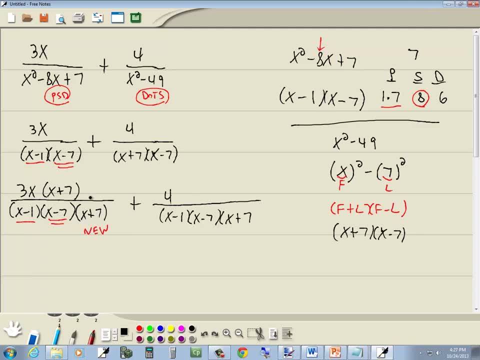 The mathematical rule behind that is: whatever you multiply by the bottom, you have to multiply by the top. In our second fraction, we have x plus 7, x plus 7 is still there. We have an x minus 7, the x minus 7 is still there. 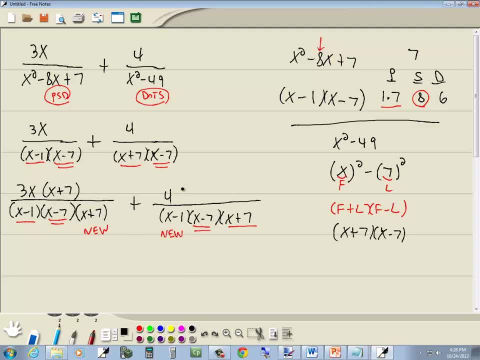 The new item downstairs is the x minus 1.. So we have to put that up on top too. Well, get rid of the parentheses up here. 3x times x is 3x squared, 3x times 7 is 21x over our denominator. 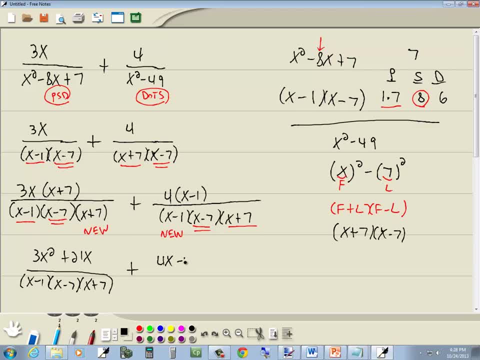 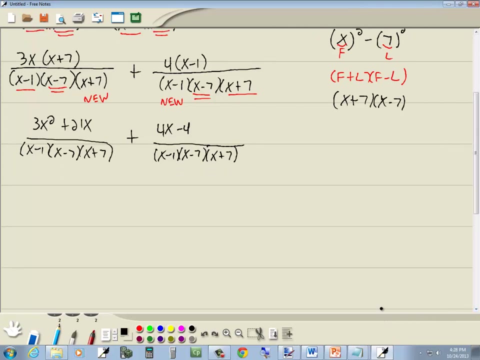 Now here we've got: 4 times x is 4x, 4 times negative, 1 is negative, 4.. Over this? Well now, since they have the same denominator, our next step says to add or subtract the top parts. So we've got 3x squared plus 21x, plus 4x minus 4..